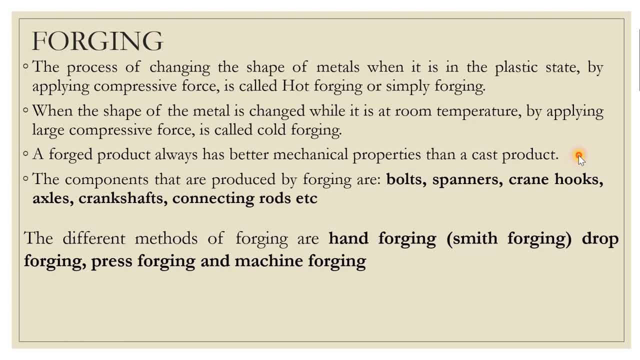 So we have three components which we're going to discuss about. Vä obliged to be」. The components that are produced using cold forging are bolt spelled, cranking hook, connect road of works that are made by using forging. So the different methods of forging are hand forging, which is also called as split forging, hand rope forging, pressure or, sorry, Press forging. 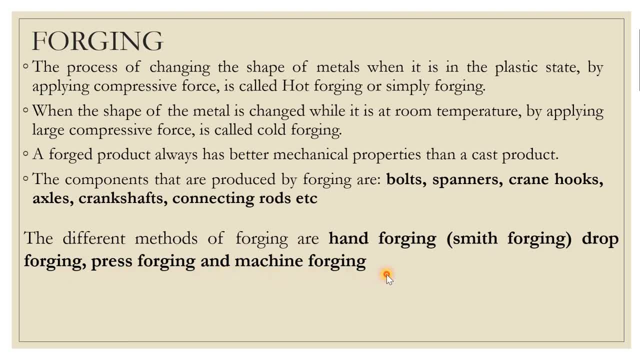 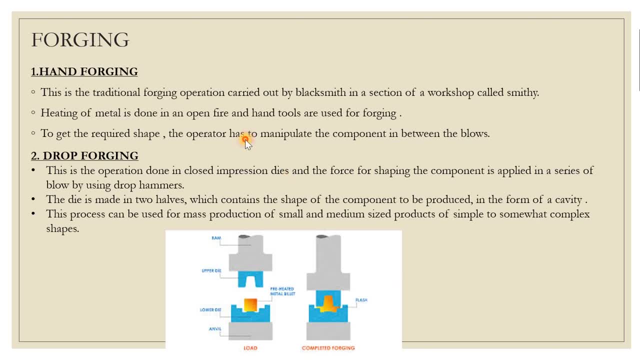 refresh forging and machine forging. so these are the different types of forging process used in manufacturers. okay, so first one: what is hand forging, so fording? there are so many types of forging and first one is hand forging. so this is the simple, traditional type of forging in which the 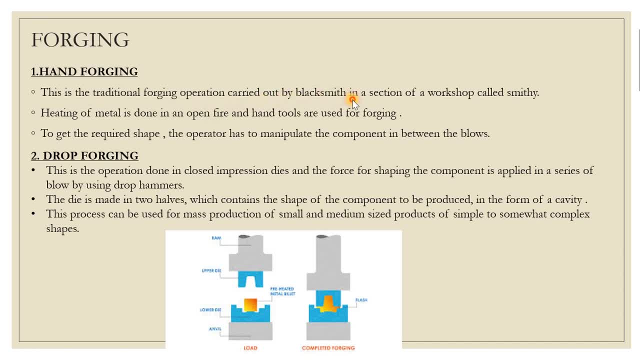 operation is carried out by blacksmith in a section of workshop called smithy, and this is carried out by blacksmith in a workshop that is called as smithy. smithy is a forging workshop. okay, so heating of metal is done in an open fire and hand tools are used. 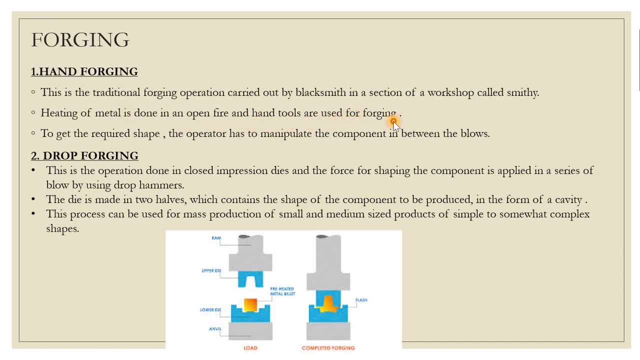 for forging. so we are operating it conventionally with our hands. okay, so we heat it with open fire. we heat it and then we forge it with our hands. we usually make knives at home like this. okay, so get the recording shape. the operator has to manipulate the component in between the bows. 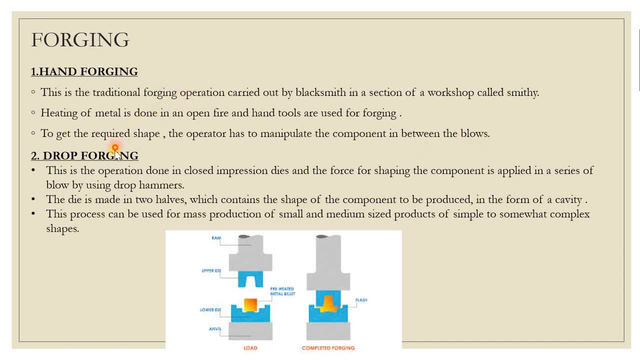 by using hand- okay, hand. and a hammer- okay. so next one is a drop forging. so this operation is done in closed compression. dies. so in this operation there is a die. so in this forging there is a die. and the die is made in two halves, which contains the shape of the component to be. 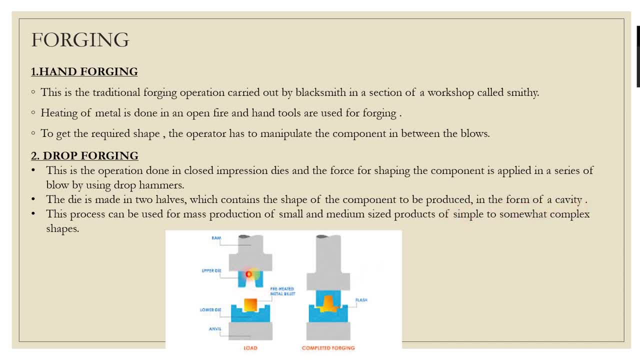 produced in the form of cavity. so what i'm looking at separately to the joint part and음 a shape of the um full body to be forged. so everything shape would have to fill out, so that is known as a drop forging. so this is operation. that in close. 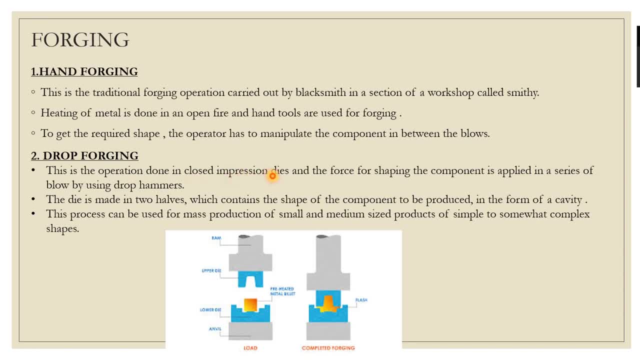 the compound dies, closed impression dies and the force for sharpening can also be形容 shaping. the component is applied in a series of bow blow by using drop hammers. a little ram wound, okay. so this process can be used for mass production of small and medium-sized production. 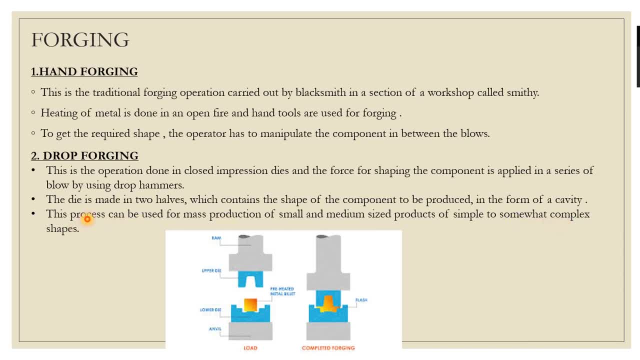 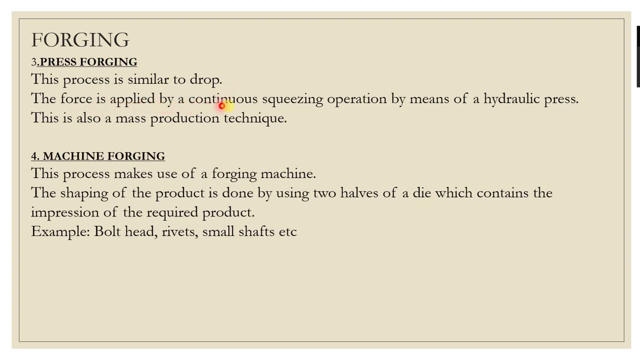 or simple to somewhat complex shape. second, one is fresh forging, so this process is similar to drop. the force is applied by continuous using operation by means of hydraulic pressure, so this is also known as mass production technology: hydraulic pressure based on the number of pressure applied. so that is the main difference. 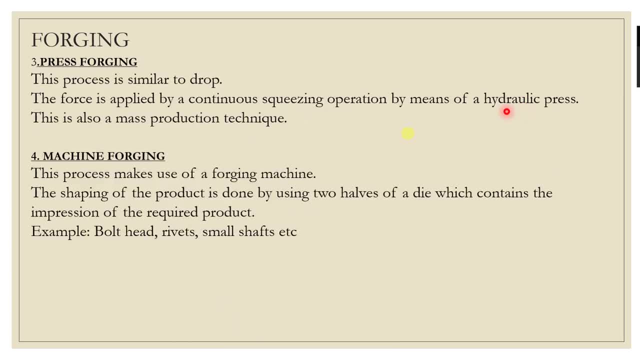 between the drop forging and press forging. okay, next one is a machine for machine forging. so this is process. this process makes use of forging machine. i'm going to use a little bit forging machine now and we are using that machine to produce forged part. okay, the shape of the product. 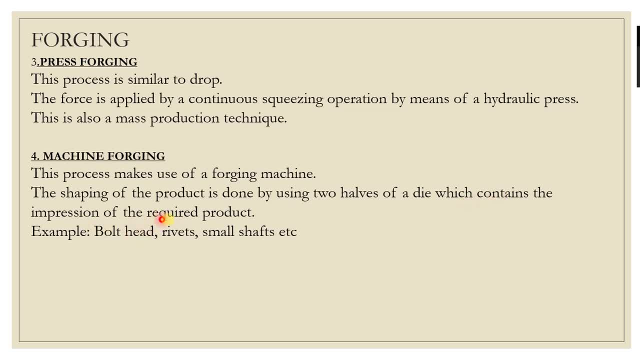 is done by using two halves of a die, which contains the impression of the required product. so examples: around the bolt head, rivet, small shaft- okay, nothing. these are the examples used to examples of the components that are machine using, machine forging: okay. so next one has hand forging operations. so there are. 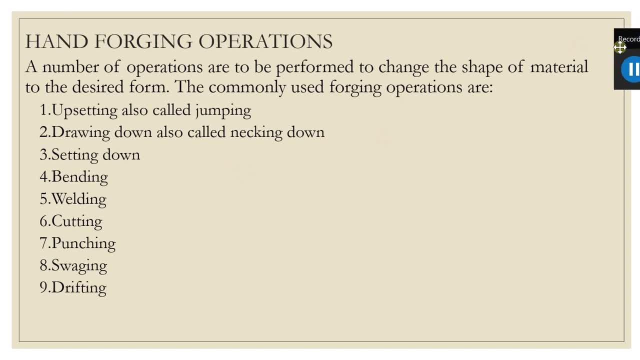 several hand forging operation commonly used in smithy operations, okay, hands off as a blacksmith, okay, a number of operations to be performed to change the shape of material to the desired form. the commonly used forging operations are: first one, one upsetting, or that is also called jumpy, and second one on drawing down. 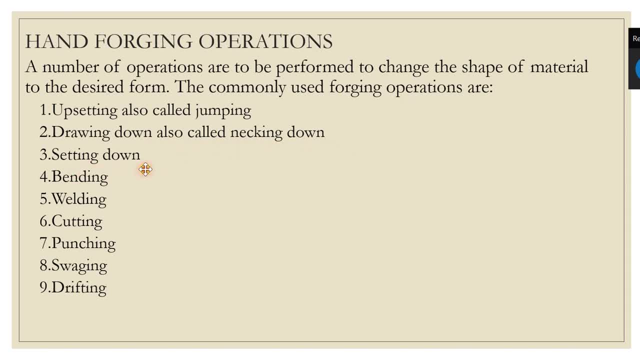 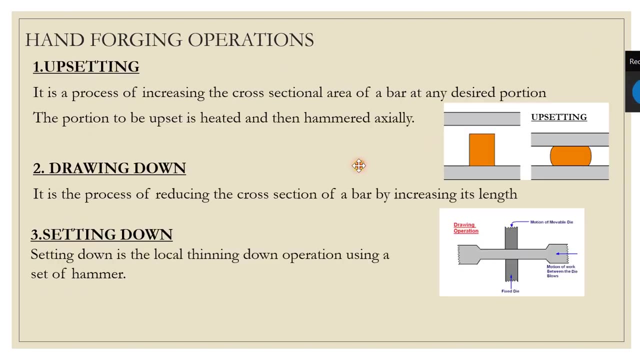 also called the necking down. and third one, sitting down. fourth, bending, welding, cutting, punching, swagging, drifting. ok, so what are these? product process, lets see. so, in upsetting operation, we are increasing the size of the desired part by using a compressive force. so lets see. 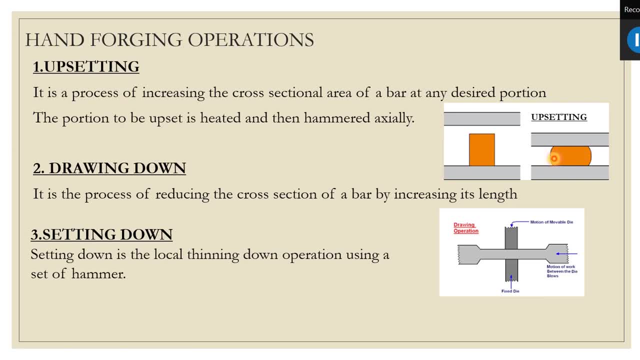 we apply a compressive force and increase the size of the cross sectional area. that is known as upsetting. drawing down is a process of reducing the cross sectional area of a bar by increasing its length. so cross sectional area small by increasing its length. setting down is a process of. 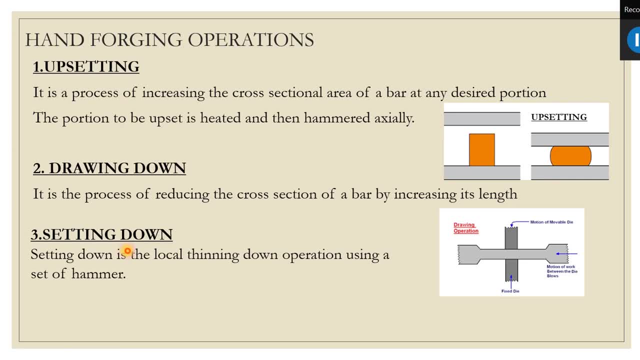 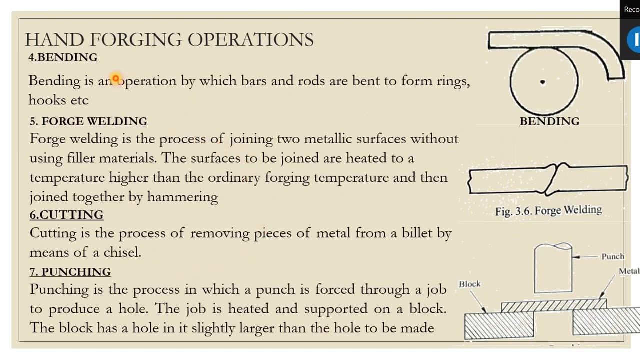 thinning the size of a particular portion. so setting down is a local thinning down operation using a set of hammer, some thinning operations in a particular part, ok, and there is bending. bending is an operation by which bars and rods are bent to form rings. so bending is bending a small bar. 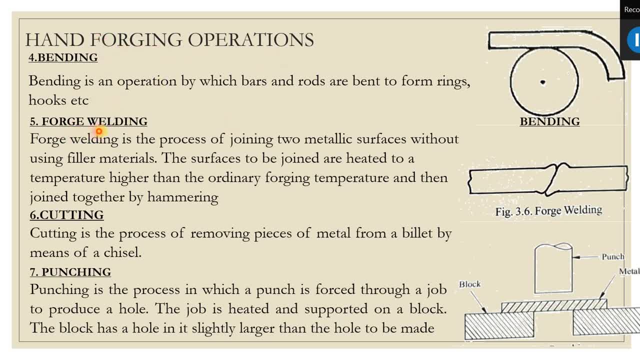 so it is also a hand forging operation. and fifth, one is a forge welding. so forge welding is a process of joining two metallic surfaces without using filler materials, so the surface to be joined are here heated to a temperature higher than the ordinary forging temperature and then joined together by hammering. 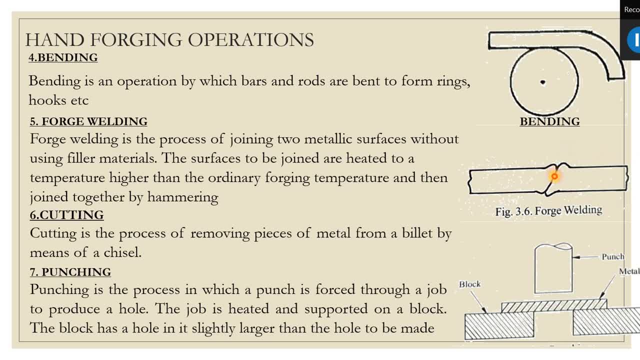 so here we are, joining the two parts by using heat and by using hammering, so by using these two parts. there is no other filler material. we heat it and then these two parts are fixed together, so that is known as forge welding. ok, and sixth one is cutting. 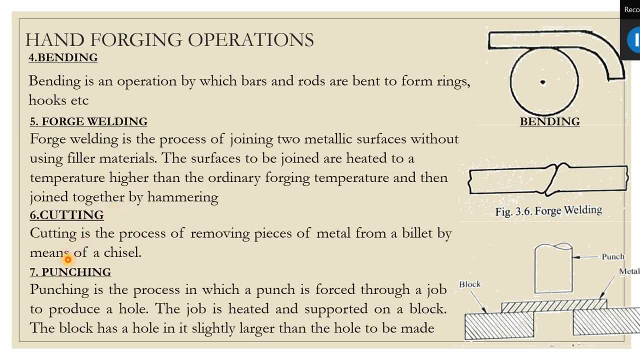 so cutting is the process of removing a piece of metal from a billet by means of a chisel and then we cut it so you notice there is not this one. so cutting is the process of cutting. so cutting operation is also a hand forging operation. and seventh one is punching. 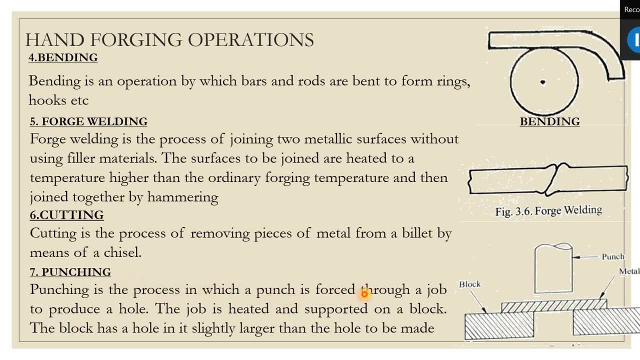 so punching is the process in which a punch is forced through a job to produce a hole. so job is heated and supported on a block so the block has a hole in it slightly larger than the hole of the hole to be made for a small part. this is the metal part. 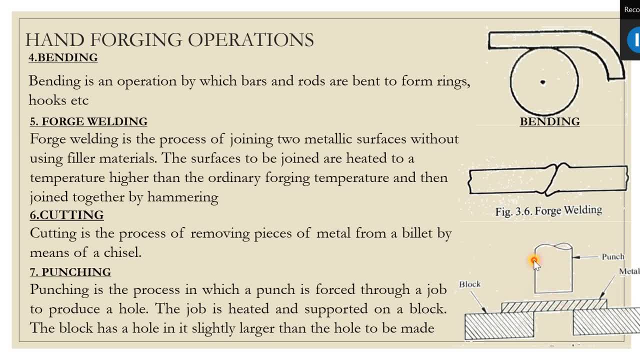 and the hole inside. it is called punching. so punching is called punching die, so punching die. we place the metal part on top and place two blocks below it. this block has a small hole. so the hole in the block, the block has a hole. it is slightly larger than the hole of the hole to be made. 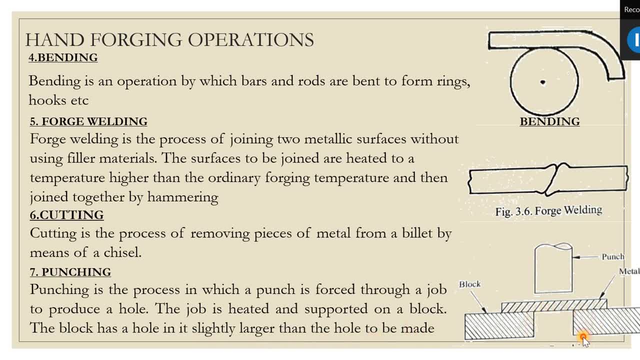 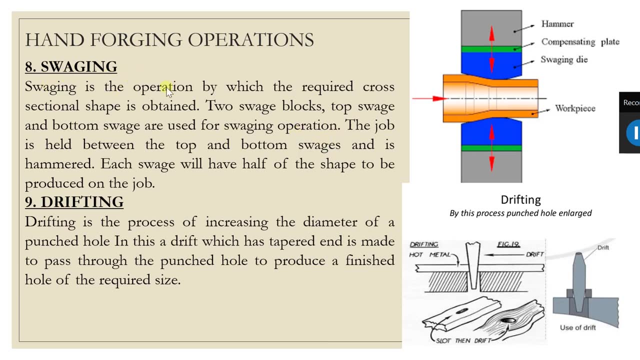 the hole we are making will be slightly larger. the width of this hole or the diameter of this hole will be slightly larger than the hole of the hole to be made. so that is the punching operation. next one is the swagging operation. in this the work piece is placed between: 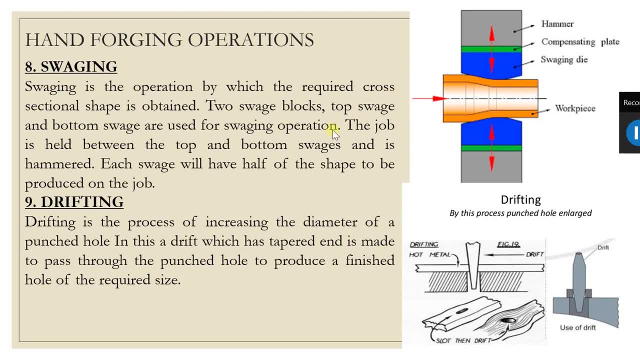 a top swag and a bottom swag and applying pressure by using a hammer, and the required shape is produced by using this two swagging dies, which is in the shape of the part to be created. so the job is held between the top and bottom. 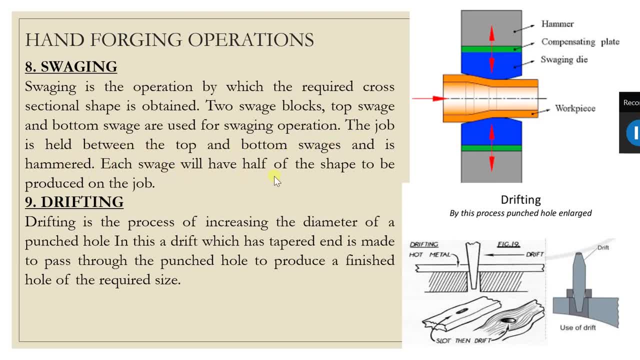 and this hammer. each swag will have the half of the shape to be produced on the job. so that is the swagging operation. another one is the drifting. so drifting is the process of increasing the diameter of the punched hole, the already intact hole. the diameter increases. 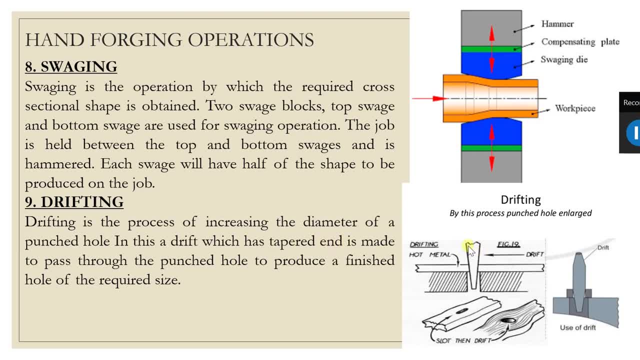 so in this, a drift which has a tapered end drifting around the tapered end area and is made to pass through the punched hole to produce a finished hole of the required size. because of the size of the tapered end, when it passes through the punched hole, the diameter of the hole will increase. 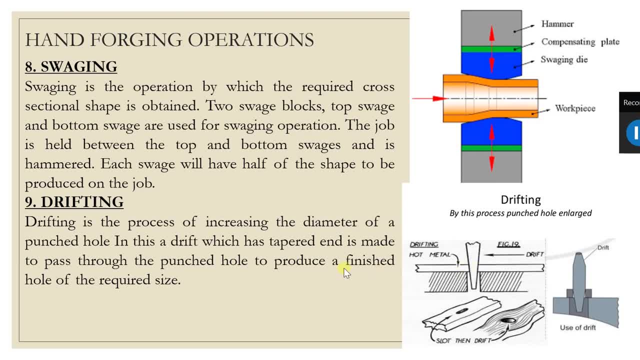 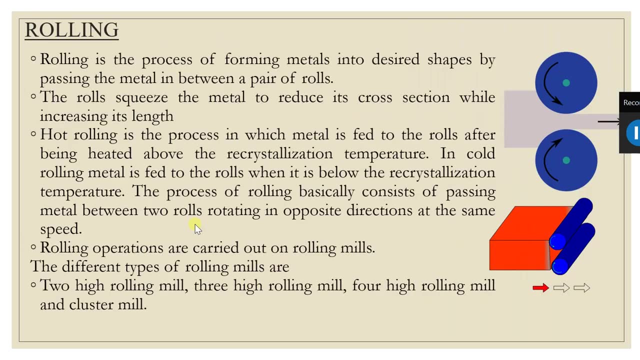 it will increase the diameter of this hole. that is what we need. so next one is the rolling. so we already completed this hand forging operations and the next operation or manufacturing process is rolling. so rolling is the process of forming metals into desired shape by passing the metals. 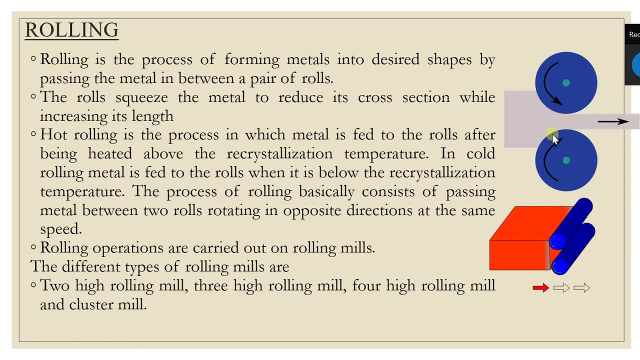 between the pair of rolls. so here we have a work piece and it is made to pass through these two rolls. so when we go inside we can see the diameter is small. sorry, the width is small. when we go inside the work piece will heat up and pass through it. 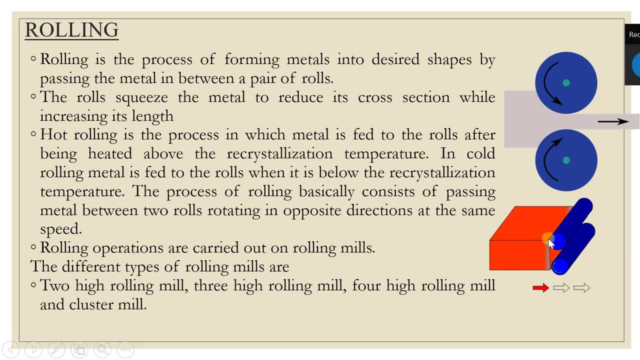 the rolls squeeze the metal to reduce its cross section while increasing its length. the length increases and the thickness decreases. so hot rolling is the process in which metal is fed to the rolls after being heated above the recrystallization temperature. so the temperature increases and in hot rolling, 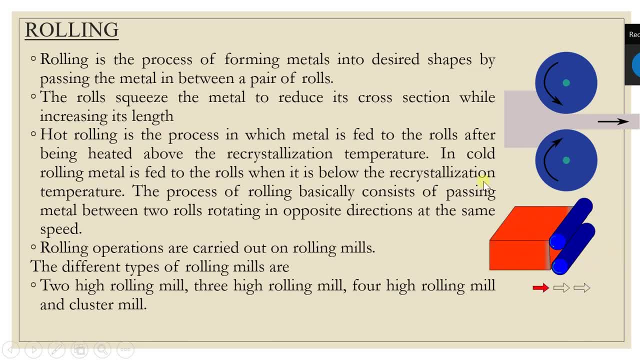 the material passes through the rolls. so in cold rolling metal is fed to the rolls when it is below the recrystallization temperature. so the process of rolling basically consists of passing metal between the two rolls in opposite direction, at the same time, at the same speed. 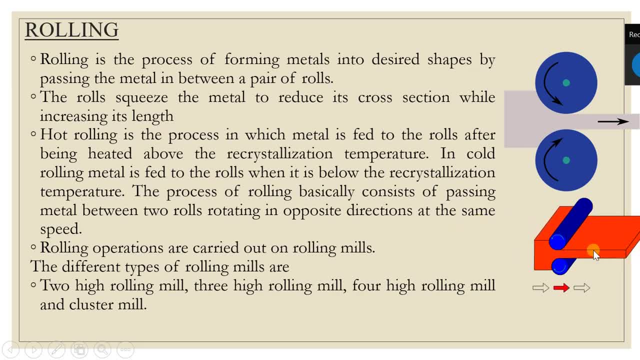 so when we pass the metal between the two rolls, its size decreases. so that is the basic idea of rolling. so we are reducing the size or thickness of the material by passing through, by passing through two rollers. so rolling operations are carried out on rolling mills, so in rolling mills. 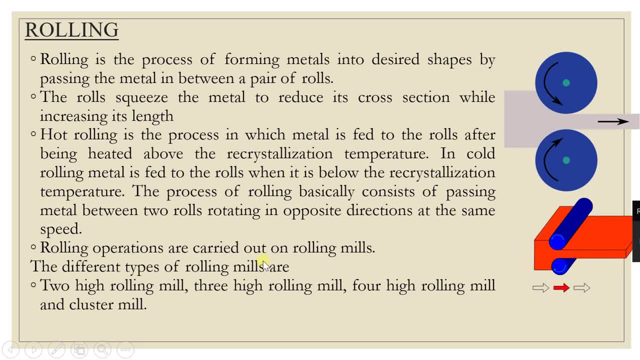 we carry out rolling operations and there are mainly four types of rolling mills. first one, two-hair rolling mill, three-hair rolling mill, four-hair rolling mill and cluster mill. these are the four main important rolling mills available. so first one, two-hair rolling mill. 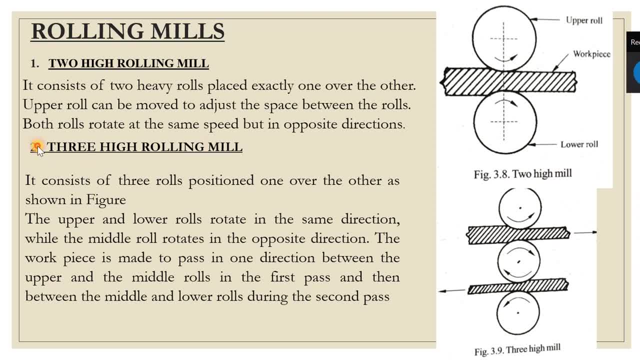 so two-hair rolling mill in earth. so it consists of two heavy rolls in earth. it doesn't heavy rolling rolls at all. first one is known as upper roll and the lower one is known as lower roll, and the work piece is mainly made to roll between. 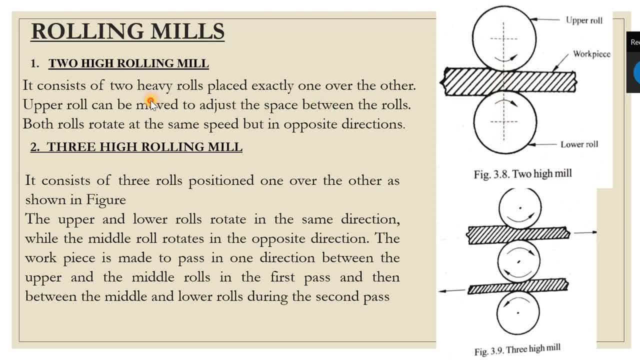 these two rollers. it consists of two heavy rolls placed exactly one over the other. upper roll can be moved to adjust the space between the rolls, to adjust the space between the rolls, upper roll moves from top to bottom so both rolls rotate at the same speed but in opposite direction. 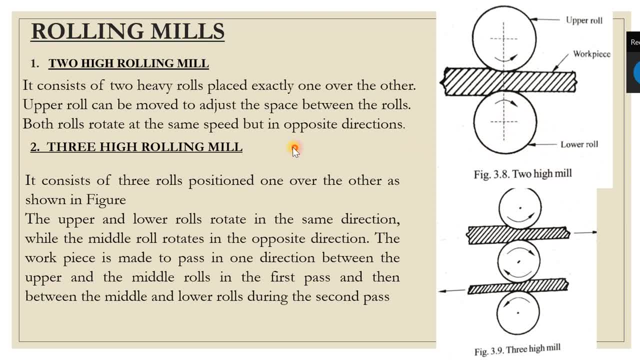 both are rotating at the same speed but in opposite direction. that is two-hair rolling mill and second one is three-hair rolling mill, so both rolls rotate at the same speed. both top three rolls are positioned in one over the other as shown in figure. the upper and lower rolls rotate in the same direction. 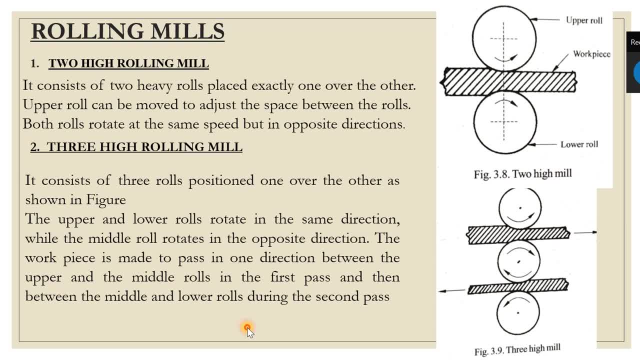 while the middle roll rotates in the opposite direction. the work piece is made to pass in one direction between the upper and middle rolls in the first pass and then between the middle and lower rolls during the second pass. so in first pass it moves up like this in second pass: 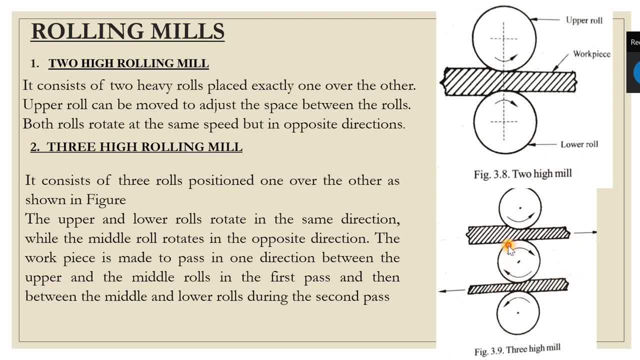 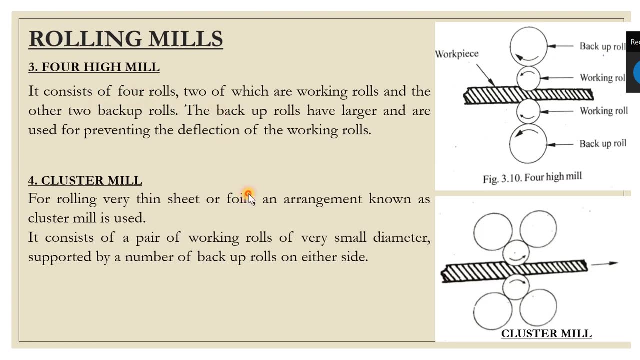 it moves two rollers below. so it moves two rollers below. the thickness is to be reduced. first pass through this and then pass through the second one, that is known as three high rolling mill, and another one four high rolling mill. so it can serve four roles, two of which are working roles and the other two 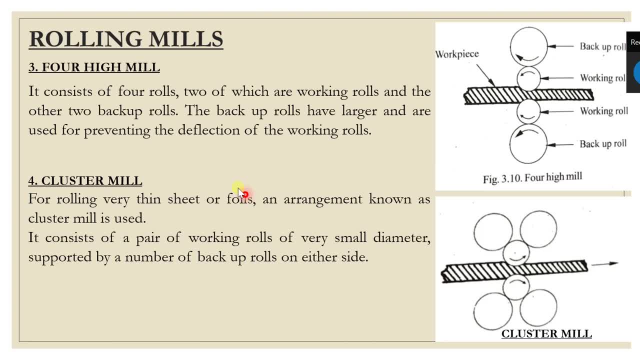 backup roles. so the backup roles have larger and are used for preventing the deflection of working roles. okay, so this is known as the deflection of working roles, to prevent the deflection of working roles. so in the background rolls the larger the working role. so working role is mainly attached to this work piece. 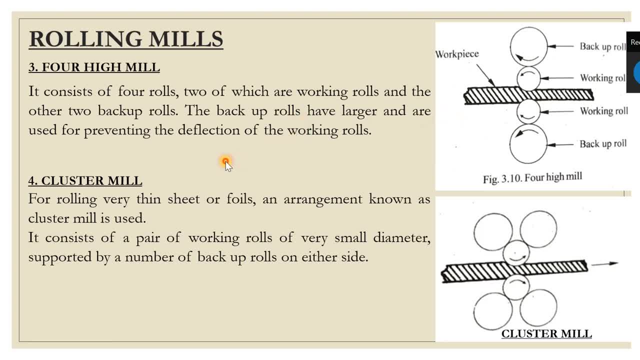 that is, four high rolling mill and the cluster mill for rolling very thin sheets of oils and arrangement known as cluster mill is used. so it consists of a pair of working roles of very small diameter supported by a number of backup roles on each side, So we are using this to make a very thin job circuit. 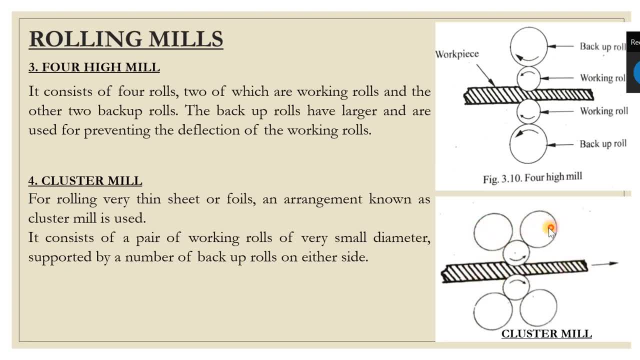 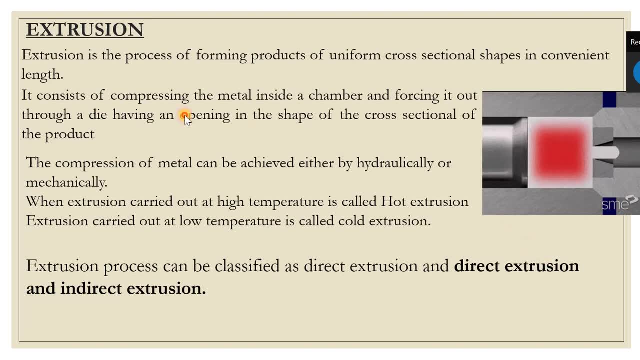 To support this, there will be two backup roles in each of them. So this is cluster mill. So next one is a very important type of process. It is called extrusion process. So extrusion is the process of forming products of uniform procession shape in convenient length. 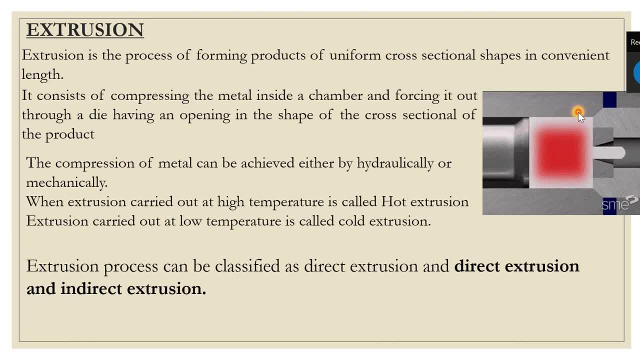 So you can understand by looking at it. Here we are passing through a small hole in a liquid or heated material. A thin sheet or a thin rectangular section comes out. So that is extrusion process. So it consists of compressing the metal inside a chamber and forcing it to out through a die. 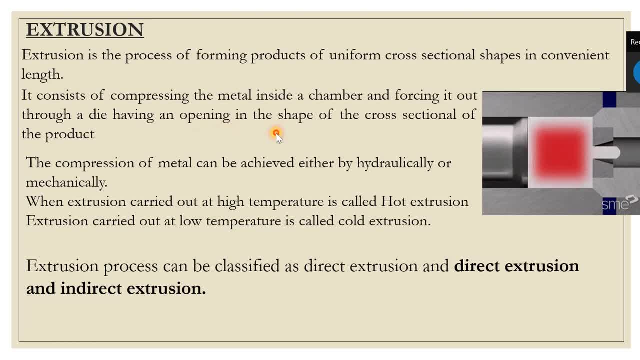 This is known as die Having an opening in the shape of a die For the procession of the product. So we have to get the die or material of opening in the shape of a die. The compression of metal can be achieved either by hydraulically or mechanically. 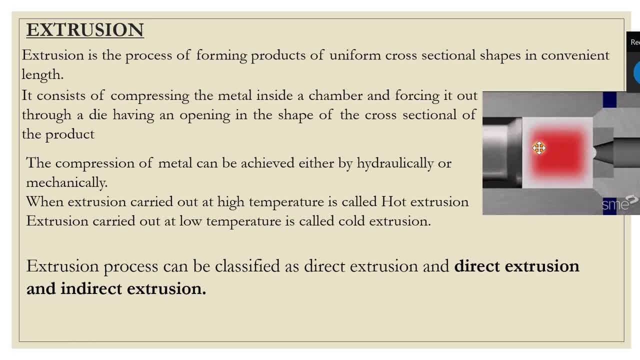 We can either compress it hydraulically or mechanically. So when the extrusion carried out at high temperature, it is called hot extrusion. So if we compress it at high temperature it is called hot extrusion, And when the extrusion carried out at low temperature it is called cold extrusion. 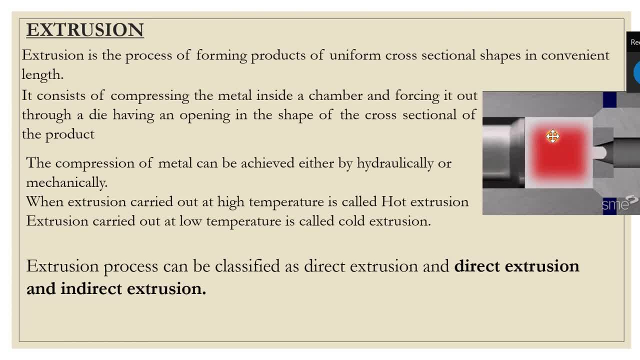 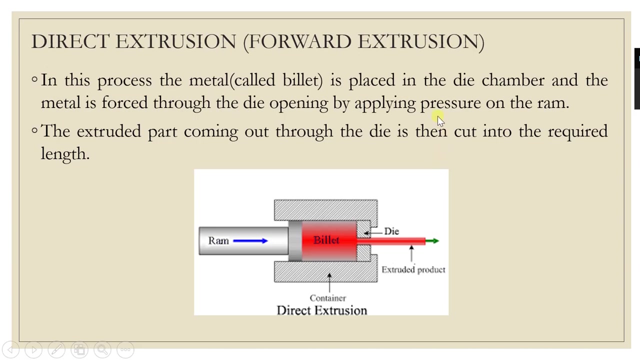 So if we compress it at low temperature, it is called cold extrusion. Anyway, we will get the cross section in this shape. So extrusion process can be classified as direct extrusion and indirect extrusion. So first one is direct extrusion process, which is also known as forward extrusion. 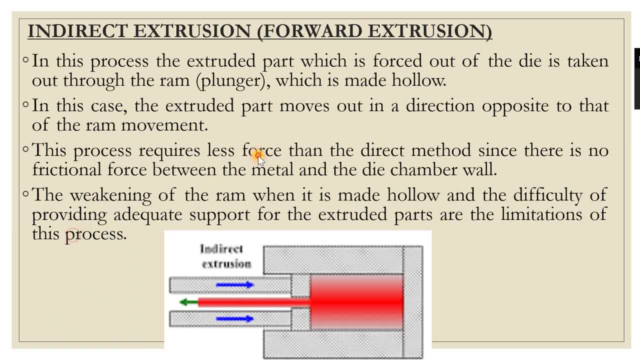 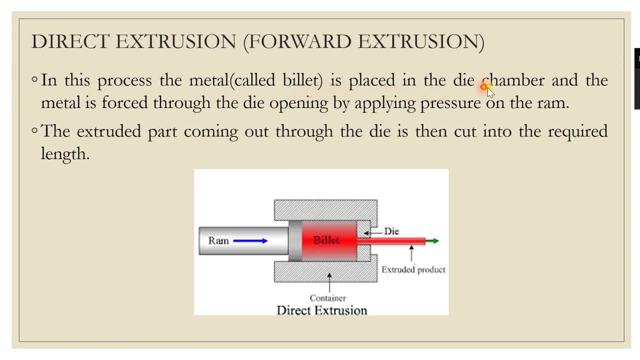 So in this process, the metal, which is also known as billet, is placed in the die chamber And the metal is forced through the die opening by applying pressure on that. We have a die chamber now, So this is known as die chamber. 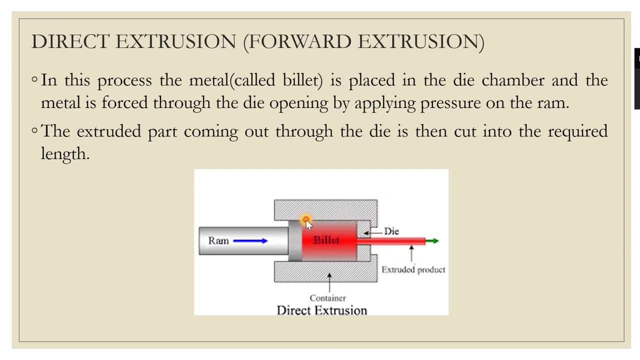 We pour the die chamber into the metal or billet And the extruded part coming off to the die And then cut into required length. We use a ram to force it. So what will happen? This small die will be of a particular shape. 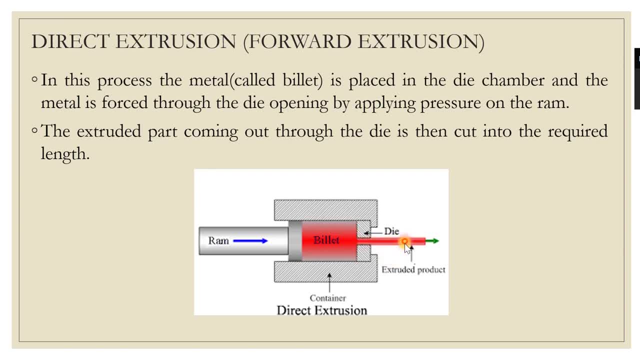 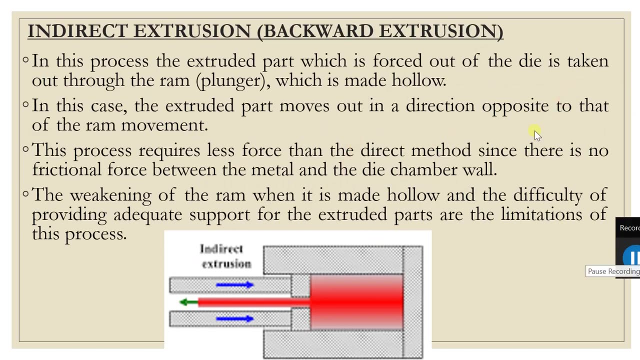 And it will come out like this. So we are cutting this extruded part in desired length. So that is direct extrusion, which is also known as forward extrusion, And the second one is indirect extrusion. This is also known as backward extrusion. 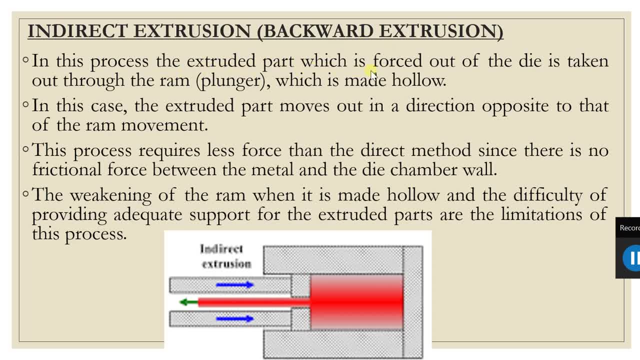 So in this process, the extruded part which is forced out of the die is taken out through the ram, Which is also known as plunger, Which is made hollow. We will fill this completely And we will do it using two rams or a simple ram. 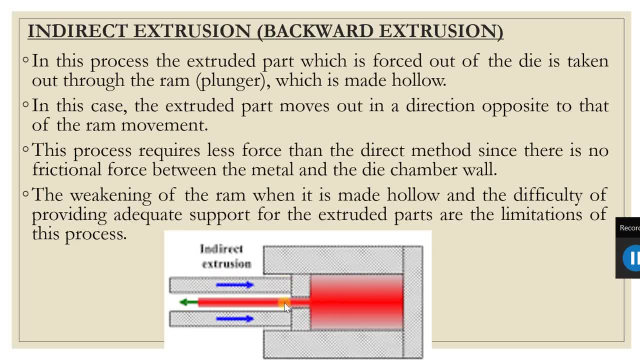 The center of this ram itself will be of desired shape. So when we force it, this part itself will come out. As we said earlier, the part on the opposite side will come out through the die. The part inside the ram itself will come out through the hole. 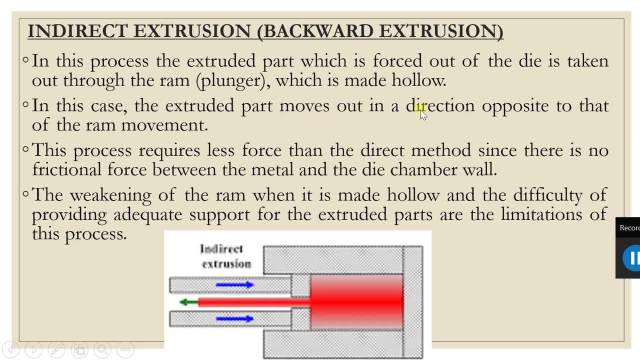 In this case the extruded part moves out of the inner direction, opposite to the ram movement. This process requires less force than the direct method, since there is no frictional force between the metal and the die chamber. So there will be no frictional force between the metal and the die chamber. 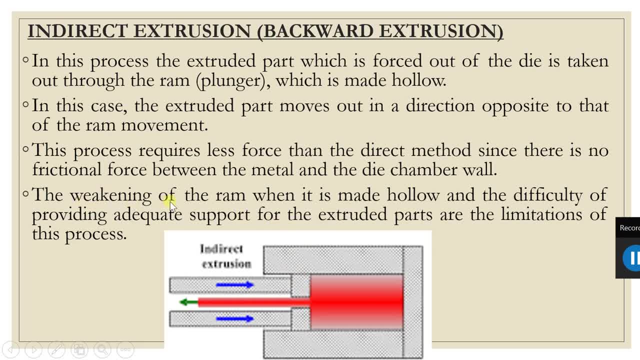 So the weakening of the ram when it is made hollow and the difficulty of providing adequate support for the extruded part are the limitations of this process. So the problem here is that the force we give is in the same direction Or the extruded part comes out through the other side. 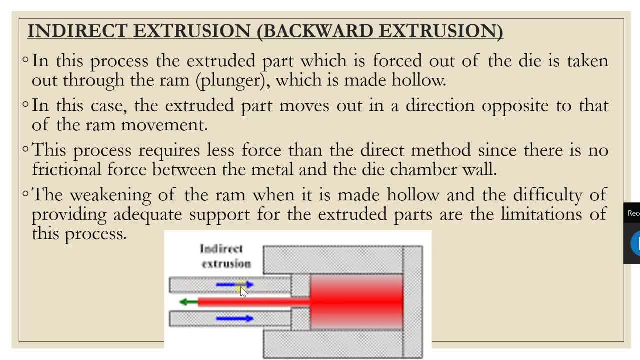 So there is a difficulty in handling it. Not only that, because there is a hole in the center of the ram, the force of the ram weakens. So these are the two main disadvantages or limitations in this indirect extrusion process. 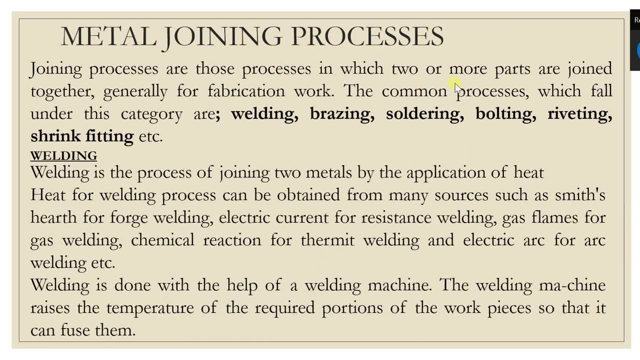 So another important manufacturing process is the metal joining process. So we are joining two metals together. So joining process are those processes in which two or more parts are joined together, generally for fabrication works. So the common processes which fall under this category are welding, bracing, soldering, bolting, riveting and string forging. 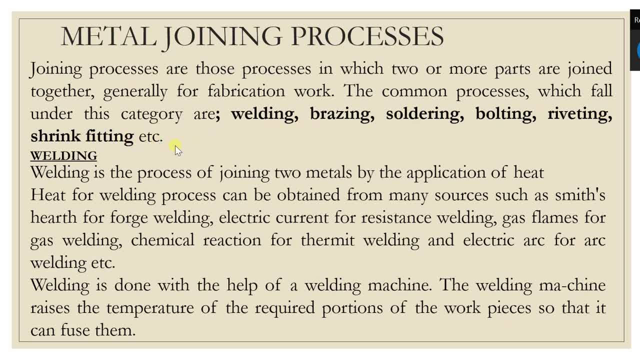 So the first one is welding. So you have already heard about welding, And welding is the process of joining two metals by application of heat. The process of joining two metals by applying heat is called welding, So the heat for welding process can be obtained from many sources. 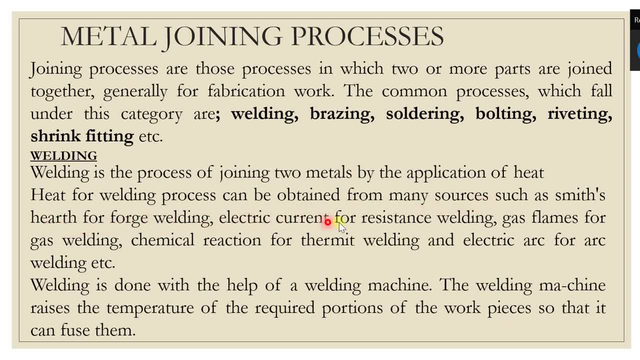 Such as smith's heart for forge welding, electric current for resistance welding, gas flames for gas welding, chemical reaction for thermit welding And electric arc for arc welding. So a heat source is there, So the heat source melts the metal. 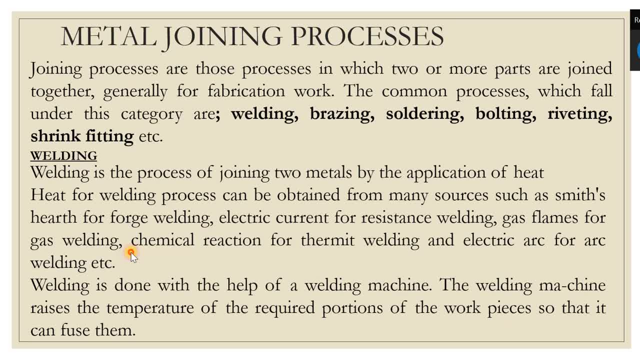 And a filler metal melts the metal And these two are joined together. So that is the main idea behind welding process. So welding is done with the help of welding machine. The welding machine raises the temperature of the required portion of the work piece so that it can fuse them. 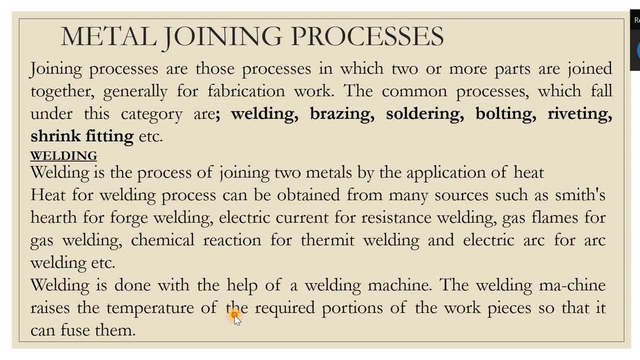 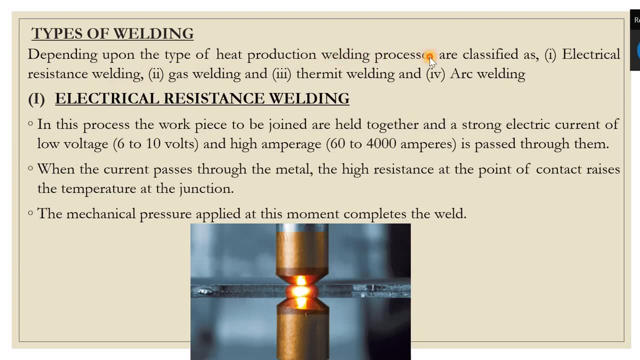 It is heated in a particular part And then it is welded. So that is the basic idea of welding. So what are the types? Depending on the type of heat production, welding process are classified as electric resistance welding, gas welding, thermit welding and arc welding. 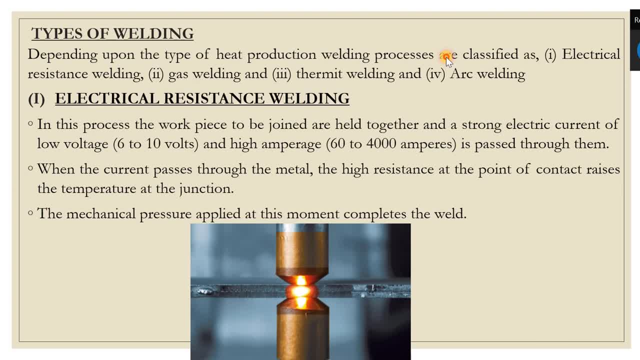 So these are the main classification of the types of welding. So how the heat is produced in the welding process is classified accordingly. So let us see what is electric resistance welding? So in this process the work piece to be joined are held together and a strong electric current of voltage 6 to 10 volts and high amperes- 60 to 4000 amperes- is passing through them. 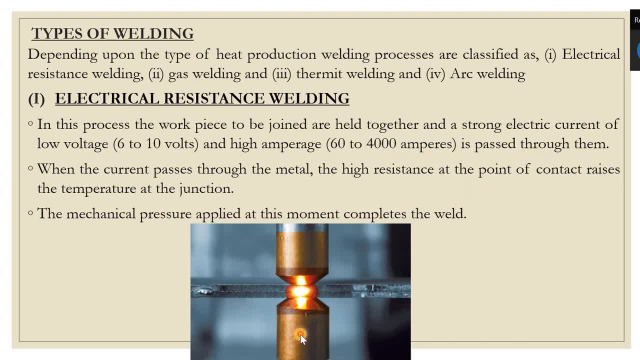 So there are two metal electrodes in it, Or the electric current passes through them. So in the meantime we are working on the work piece, So how it is done. In this joint portion there is a very high temperature. 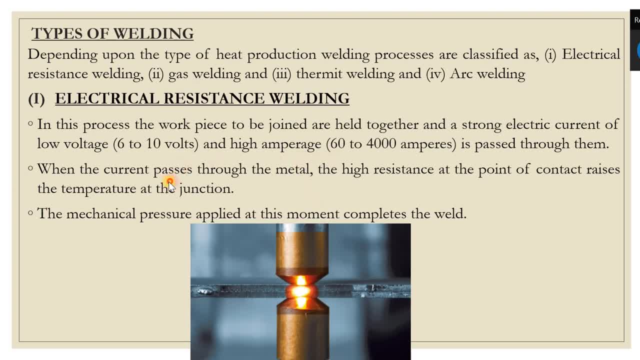 So because of this high ampere current, When the current passes through the metal, the high resistance at the point of contact raises the temperature of the junction. So the resistance at the point of contact increases the temperature Because the current passes through the high amperes. 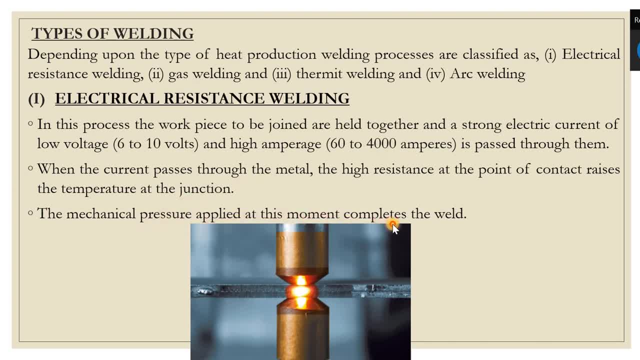 So the mechanical pressure applied at the moment completes the weld. So at the same time we are forcing both the places. Here there is a mechanical force, This hot part is fused. So that is how electric resistance welding is done. 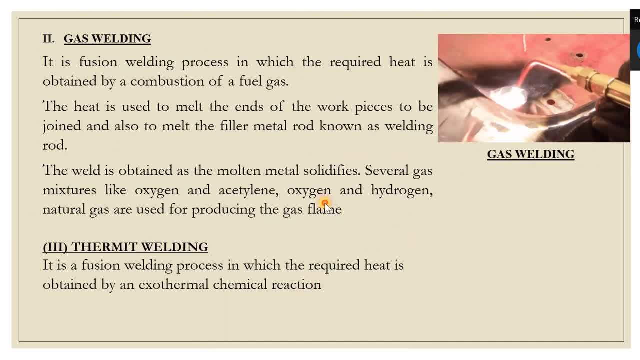 Okay, So next is gas welding. So it is a fusion welding process in which the required heat is obtained by a combustion of fuel or gas. Sorry, combustion of fuel gas. Okay, So that is what gas welding is. It is called an oxy-acetylene gas. 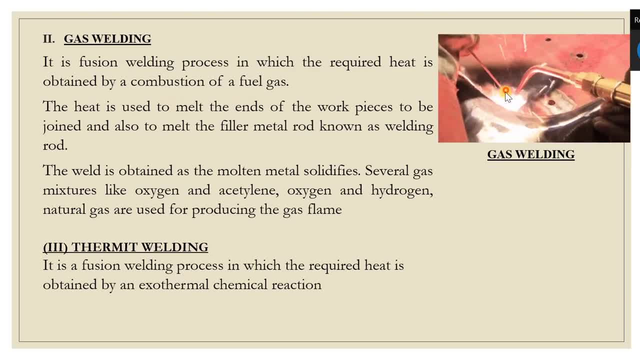 So we will burn that part. After burning that heat, We will burn that part. That is what metal is inside. So the heat is used to melt the ends of the workpiece to be joined and also to melt the filler metal known as welding rod. 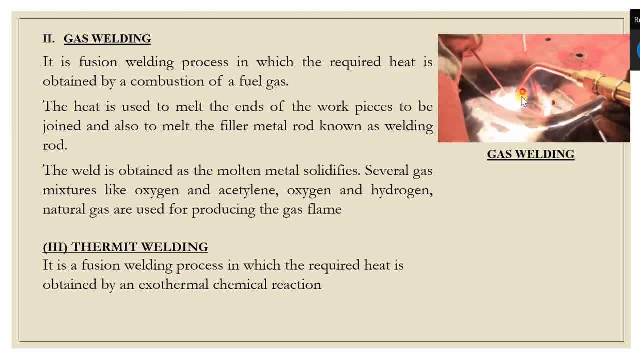 There will be a filler metal inside. This workpiece will also melt. This filler metal will also melt. After that both are fused and joined to that part. Finally, both are joined, So the weld is obtained as the molten metal solidifies several gas mixtures like oxygen and acid. 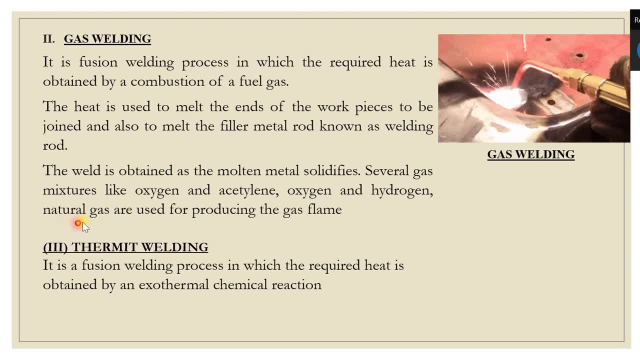 Oxygen and hydrogen natural gas are used for producing the gas flame, So the gas itself will come in When the gas is sparked. the gas will be heated or it will burn, So it will be joined to the metal or filler metal at that temperature. 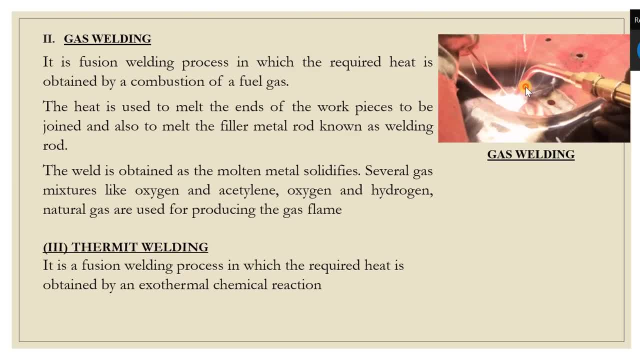 That is gas welding, So another one is known as thermit welding. So what is thermit welding? It is a new type of welding. Thermit welding is used to weld the railway lines, So it is a fusion welding process in which the required heat is obtained by an exothermal chemical reaction. 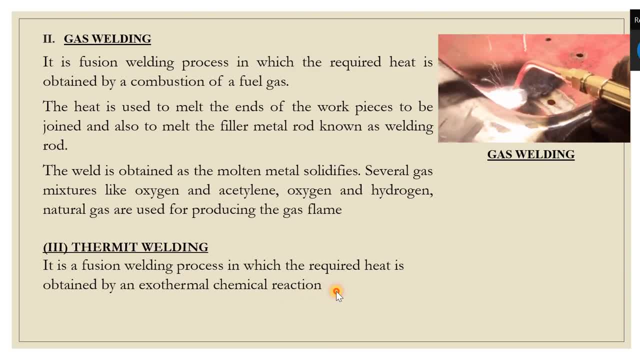 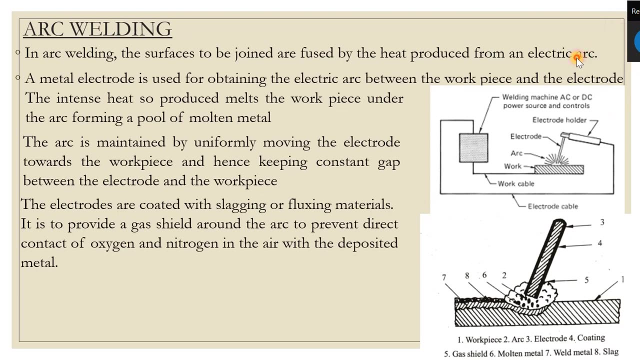 So it is used to make a railway bridge for the railway. That is thermit welding. Okay, So next one is a very important welding. It is called arc welding. So arc welding is a very important welding, So it is commonly used welding machine. 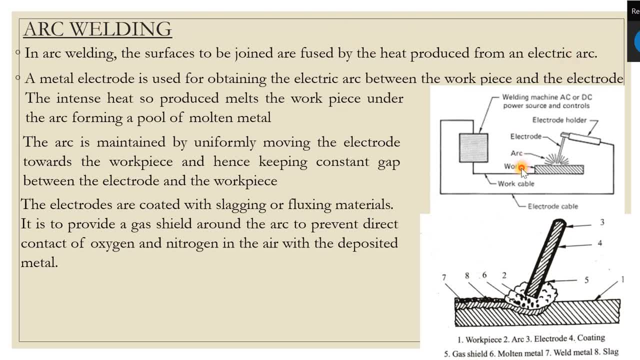 It is called arc welding machine. So here the main part is that there is an arc welding machine which is an AC or DC power source and controls. Okay, So there is a small cable coming from it That is known as work cable. 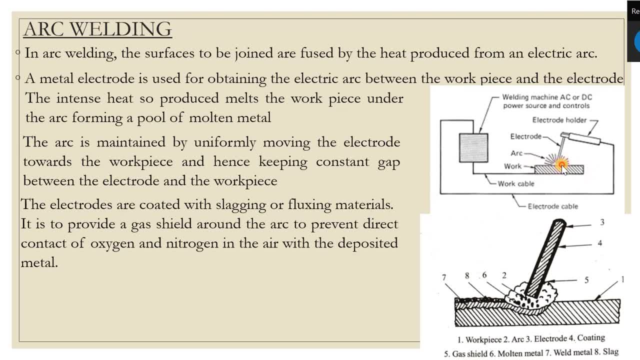 And work cable is connected to the work in which we want to make the weld. Okay, And the other part, or the next line coming from it, we pass it to an electrode by using an electrode holder. Okay, So one terminal will be positive and the other will be negative. 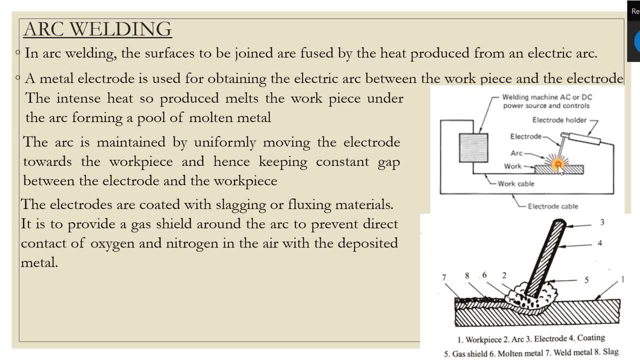 So when we mix these two together, the two will not touch each other. There will be a small gap. So through that gap, an arc will form here, Okay. Plasma arc will form here- Okay, So that arc will form here itself. 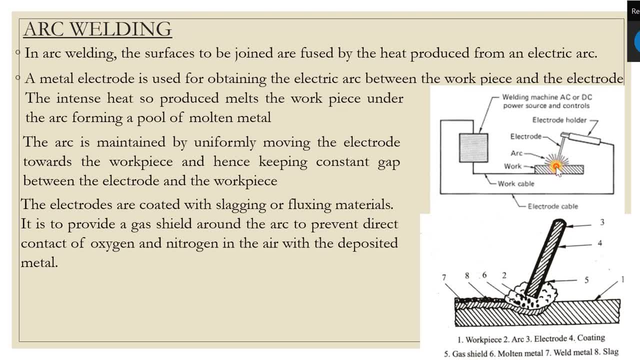 There will be a very extreme temperature rise, So the metal will melt due to that temperature. Okay, So the filler metal inside the electrode will also melt. Okay, There will be a coating outside. So that is how arc welding works. 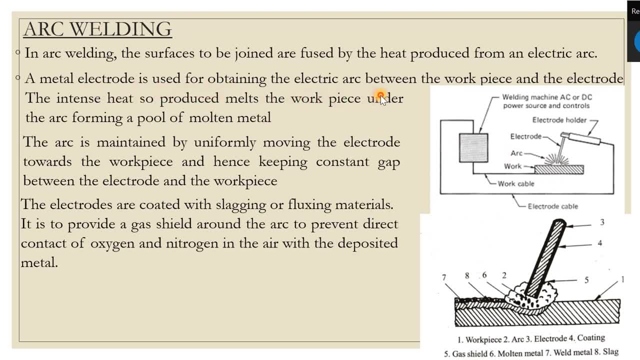 So metal electrode is used for obtaining the electric arc between the work piece and electrode. So the intense heat thus produced Melts the work piece under the arc, forming a pool of metal or molten metal. Okay, So the arc is maintained by uniformly moving the electrode towards the work piece. 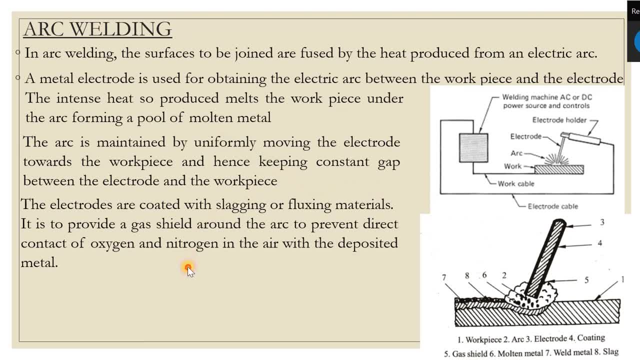 And hence keeping constant gap between the electrode and the work piece. So the amyloidic gap will be managed. Okay, The electrodes are coated with slugging or fluxing material, So coating in the electrodes and other This is used to produce a gas shield around the arc. 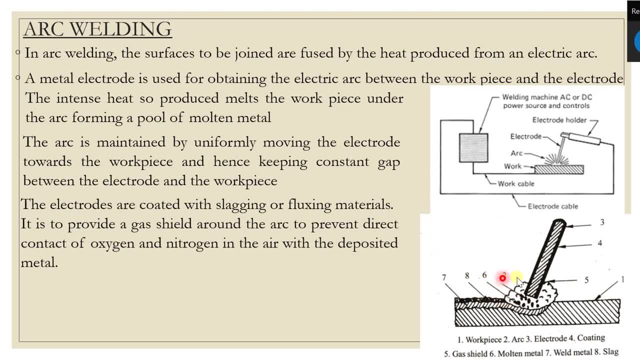 Okay, So the arc is covered and this is used to produce a gas shield around the arc. Okay, So it provides a gas shield around the arc to prevent direct contact of oxygen and nitrogen with the deposit material or metal. So, to prevent direct contact of oxygen and nitrogen with the metal deposited. 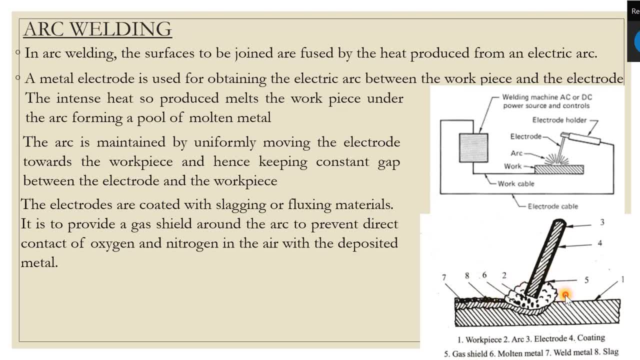 we use an arc or a coating of a gas. That is why we use the filler metal outside the electrode, Right? What do we call it? We use filler materials, We use flexing materials. Just look at the above. The first one is the work material and the second one is known as arc. 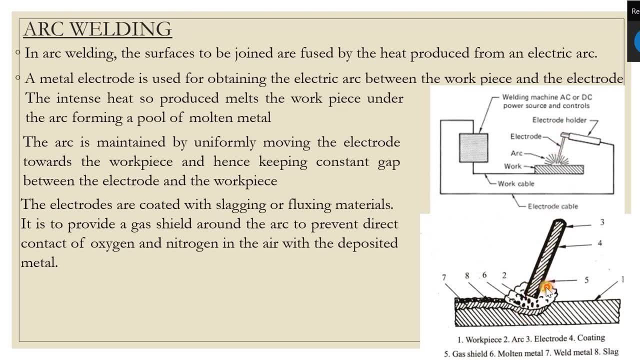 Arc is formed between the work piece and the electrode. So because of this arc, intense heat is produced at the joint. at this point This heat melts the work piece and joint them together. So the fifth one is a gas shield that comes out like this: 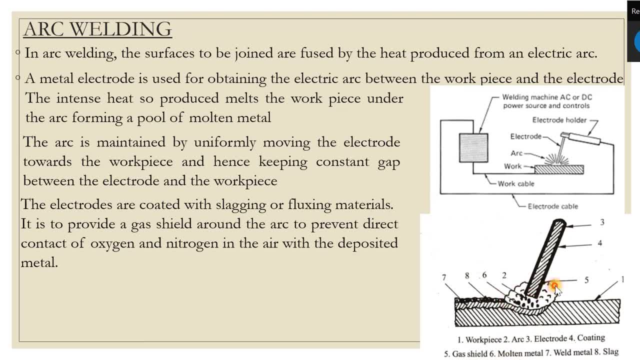 And the sixth one is called molten metal. It is the pool of molten metal. The seventh one is called weld metal. It moves like this, So this electrode moves like this, and the welding comes like this, So this is known as arc welding. 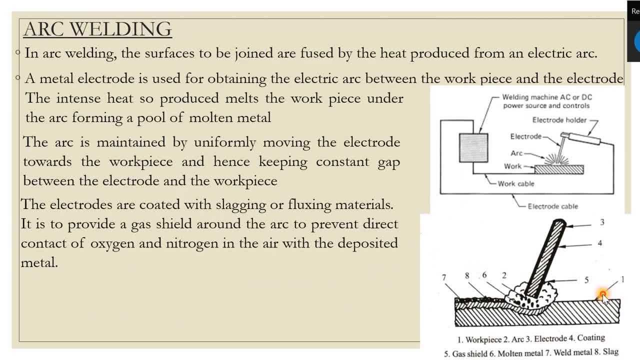 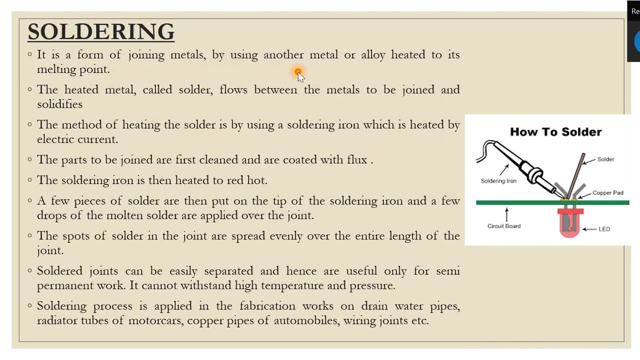 So the next one is called soldering. So it is a form of welding, It is a form of joining metal by using another metal, alloy, heated to its melting point. This is what we call soldering ions. at home We usually use soldering on electronics or electrical parts. 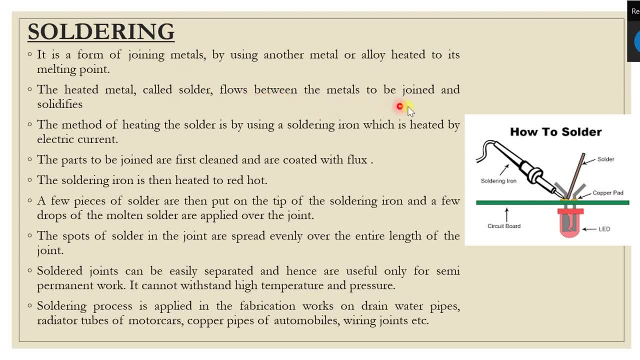 The heated metal, called solder, flows between the metal to be joined and solidifies. The method of heating the solder is by using a soldering ion which is heated by electric current. The soldering ion is heated, Then a solder is used. This solder has a very low melting point. 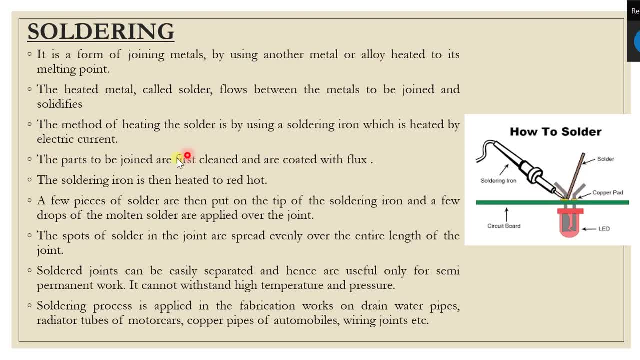 It melts here and fuses here. The parts are to be joined First cleaned and arc coated with flux. This flux is used. This soldering ion is then heated to red hot. This soldering ion will heat up well. A few pieces of solder are then put on the tip of the soldering ion. 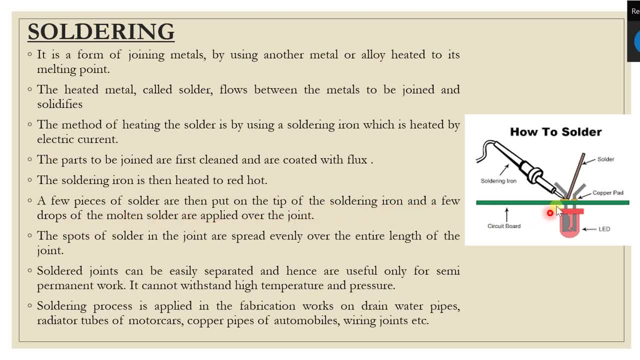 And a few drops of the molten solder are applied over the joint. We have to bring this to the tip of the soldering ion, which is hot. The spot of solder in the joint has spread evenly over the entire length of the joint, So this is given evenly everywhere. 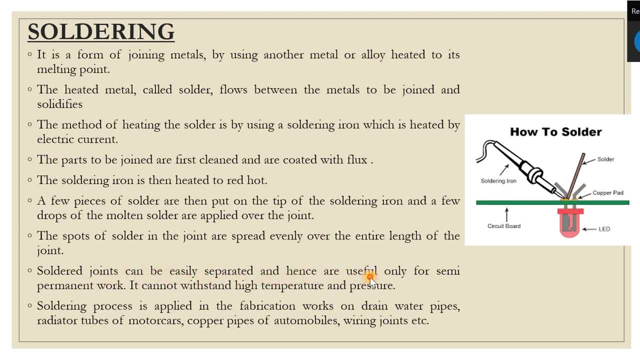 Soldering ions can be easily separated and hence are useful only for semi-permanent works. It cannot withstand high temperature and pressure. It cannot withstand high temperature and pressure. Soldering process is applied in the fabrication work on drain water pipes, radiation tubes, motor cars, copper pipes, automobiles, wiring joints, etc. 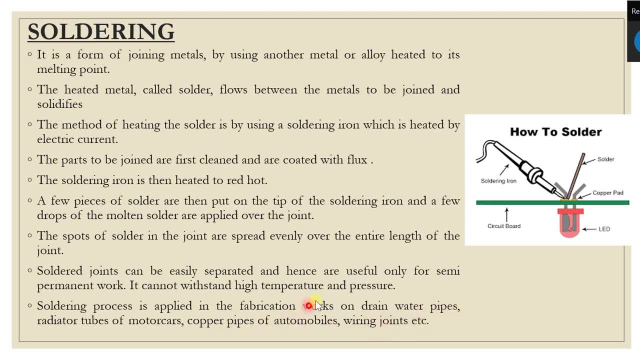 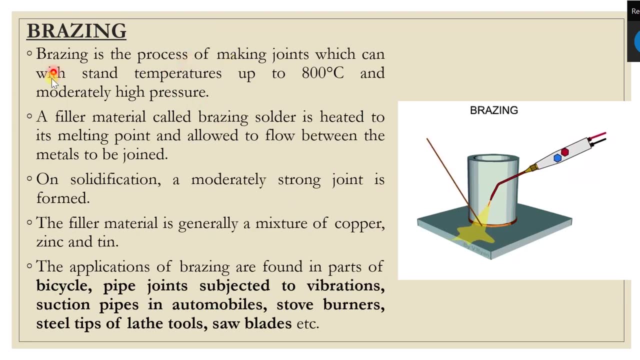 Soldering is done on the main wiring joints and other parts of the automobiles, And it is using soldering bolt or soldering ion and a solder. Okay, Next one is the brazing. Brazing is the process of making solder And it is used for making joints which can withstand temperature up to 800 degree Celsius and moderately high pressure. 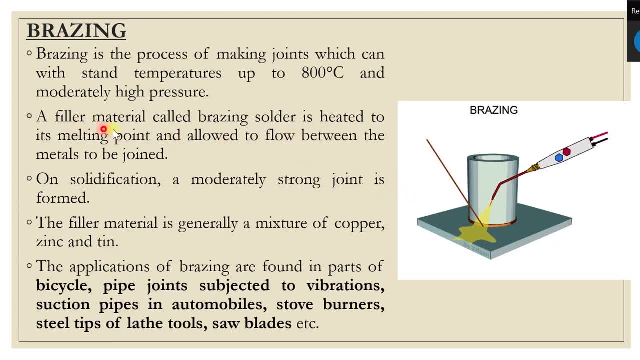 We have seen the operation of brazing compression earlier. A filament material called brazing solder is heated to its melting point And allowed to flow between the metals to be joined. That is a filament material. We are giving the temperature to it. Then it will melt and join to the joint.